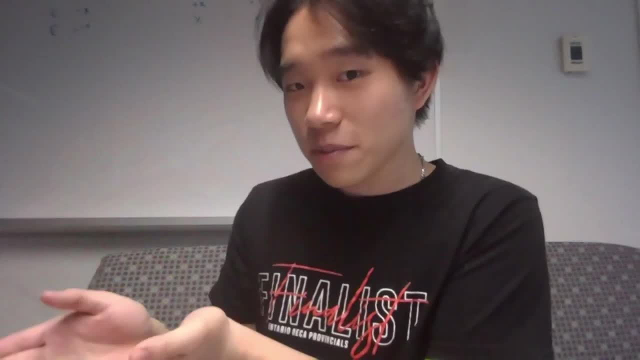 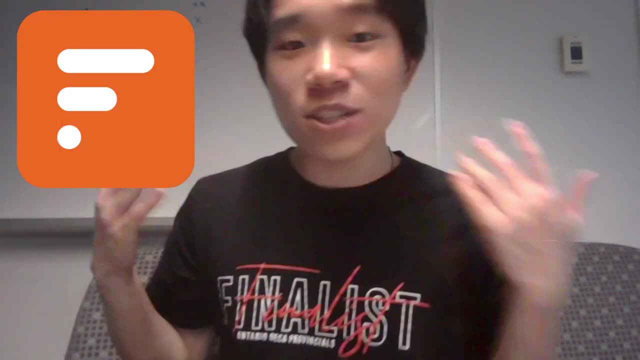 well your business is doing, and whether your business is doing better than before or worse, And so thousands of businesses actually use formula loop to create their customer satisfaction forms, and you can do that too. Starting today, make sure that you have a break from your 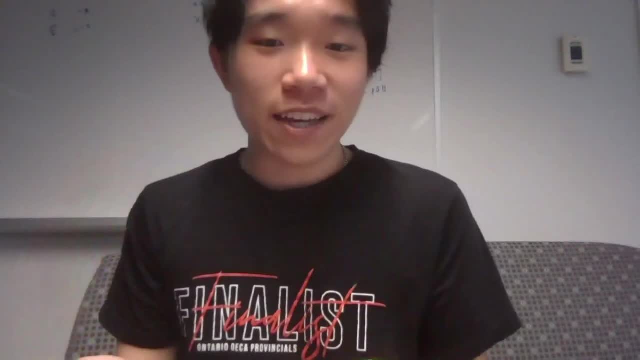 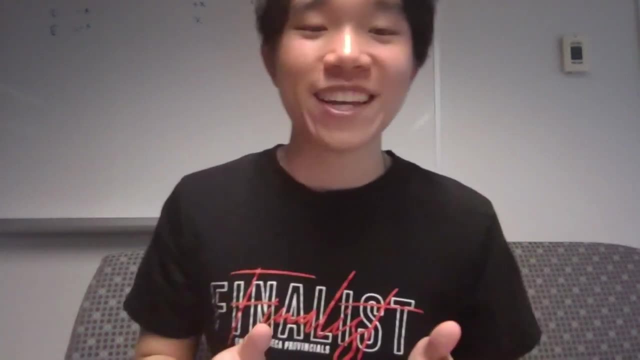 business. Take a break from your products. take a break from your products. take a break that you like and subscribe. so, before we head into the new video and let's get started, let's hop on the editor and i can show you exactly how you can create your own customer satisfaction survey. 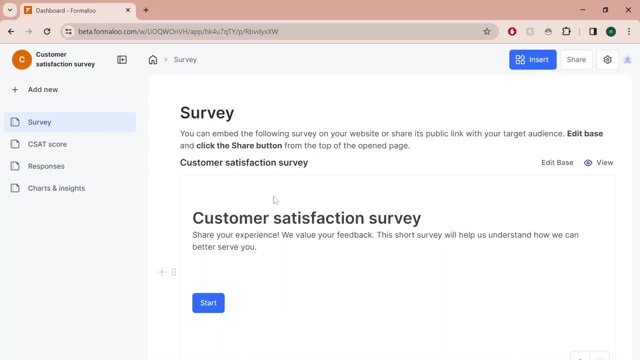 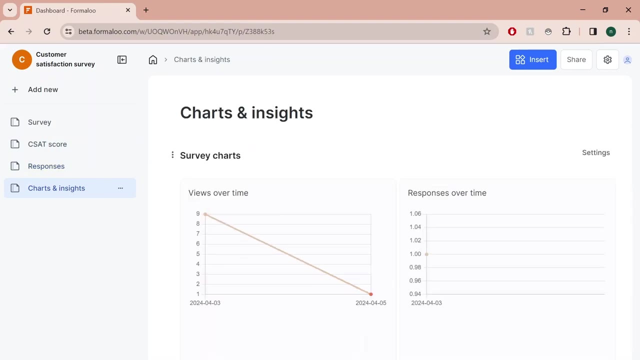 alrighty, so here we are on the editor. once you click on one of our awesome templates- the customer satisfaction survey template- it formally should automatically create you an app that looks like this, which tracks your csat score, your responses, and it also compiles your information into a chart. 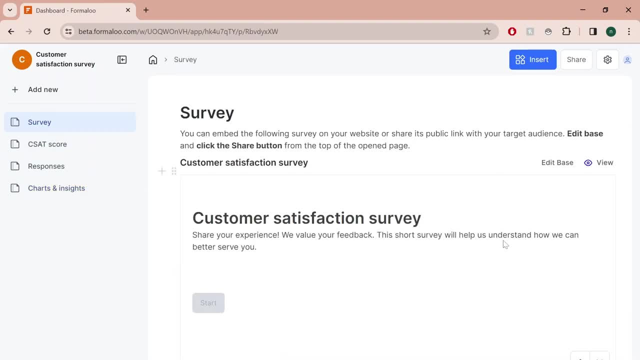 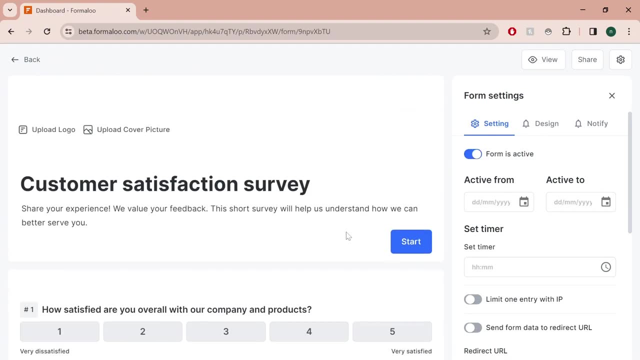 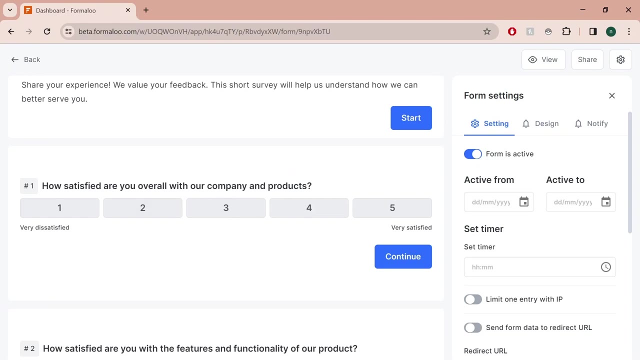 which is really cool. um, here is the survey. let's just edit the base and kind of just get into how you can create your own and customize your own survey form. so, customer satisfaction survey. you can change all the text. this change will completely upload logo. you can change the different fields. 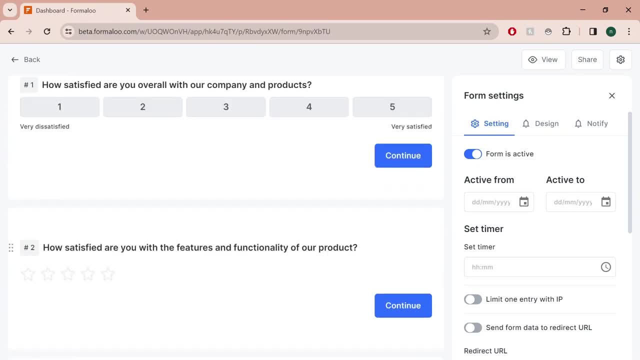 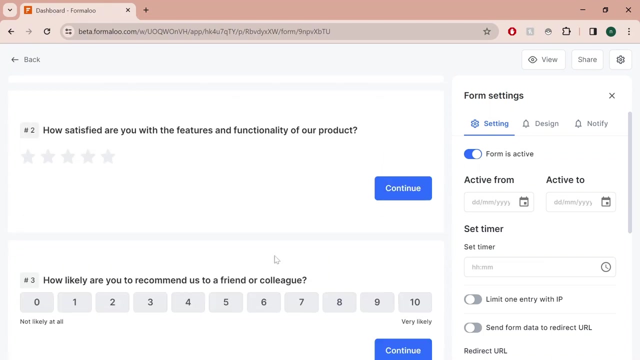 here is. obviously the most important aspect of the custom satisfaction survey is the rating scale. so you can either do through stars, which is pretty visual and pretty easy for the customer to understand, or you can just do one through five scale from very dissatisfied to very satisfied. this is kind of the bread and butter of 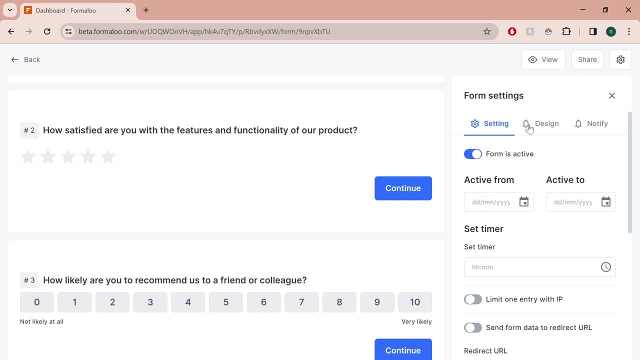 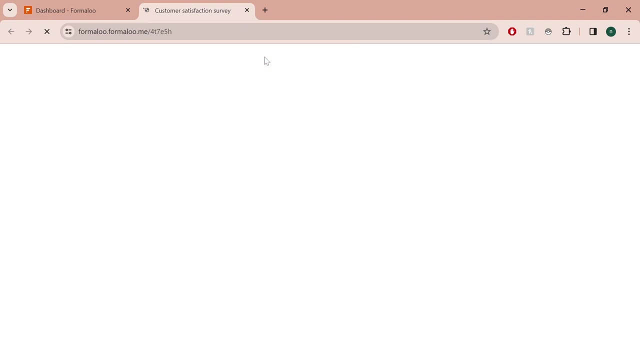 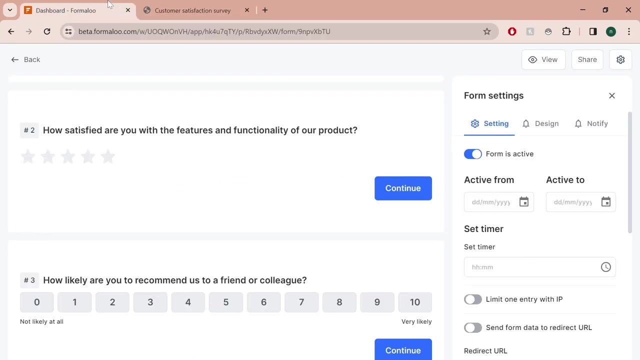 your customer satisfaction survey and so over here. form settings, you can click on design similar to our other videos have already also gone into them as well, and so notify to get notifications, obviously. view button. if you ever want to share the link with anyone, you can. all you have to do simply copy this link, copy and then paste it onto whatever email you. 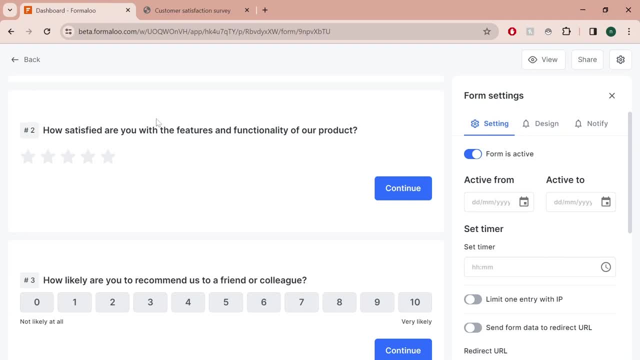 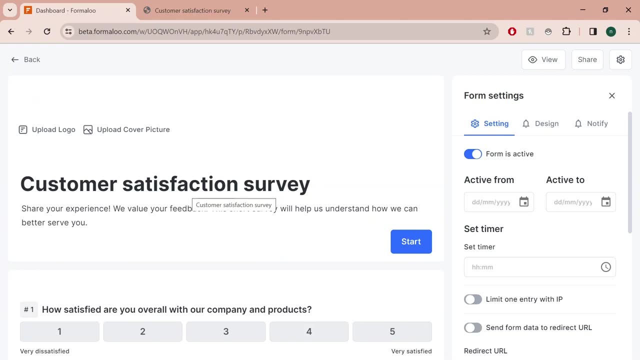 want to send to your customers or whatever company website you have. it's super easy, super quick and yeah, that's kind of it for today. a really brief summary of how you can create a customer satisfaction survey and make sure you guys like and subscribe, just to show that you guys are. 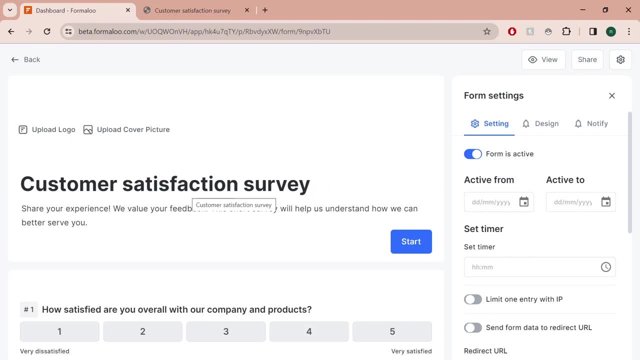 engaged in that. you guys support us and we will see you in the next ones. Bye, Hope, you guys have a great rest of your day and HAPPY PORNALOOI.